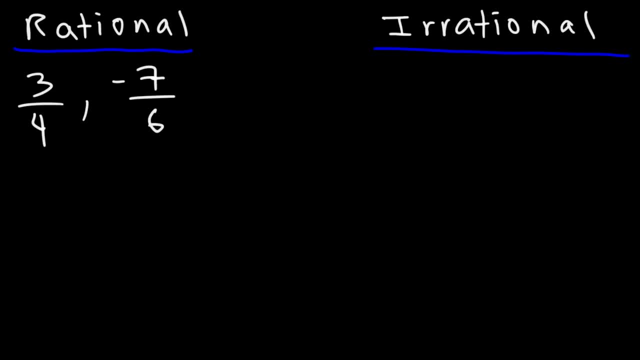 So here's a question for you: Is an integer a rational number or an irrational number, For example the integer 8.. Would you put it on a left column or on the right column? So can we write 8 as a ratio of two integers? 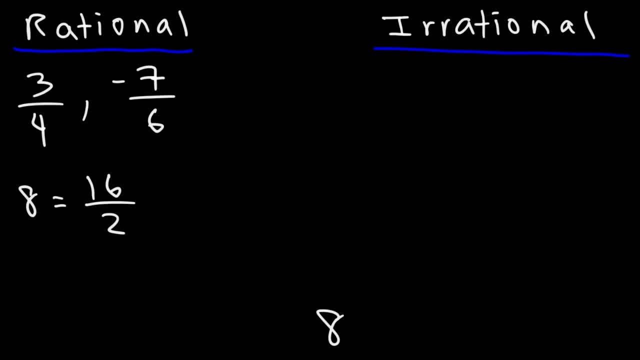 We can write 8 as 16 divided by 2.. So 8 is a rational number. What about a negative number like a negative 5? Is that a rational number? Negative 5 can be written as a ratio of two integers. 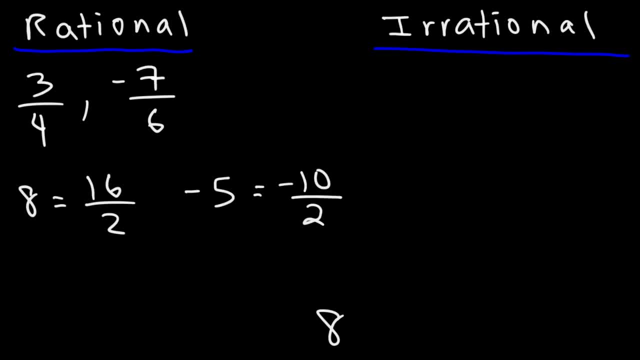 You can write it as a ratio of two integers. You can write it as negative 10 divided by 2.. So negative 5 is a rational number. In fact, all integers are rational numbers. Now what about, let's say, decimal numbers? 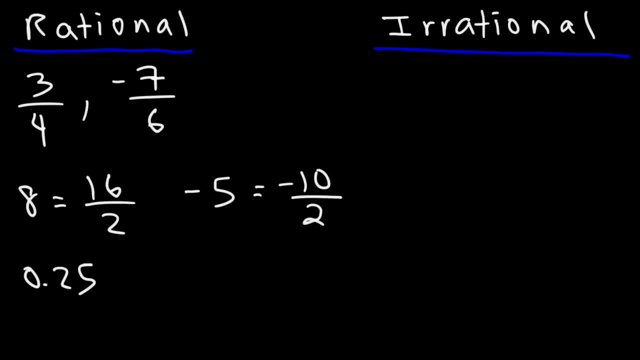 For instance 0.25.. Is that rational or irrational? Can we write this as a fraction Using two integers: 0.25 is the same as 25 divided by 100.. And if you divide the top and the bottom number by 25, this is the same as 1 over 4.. 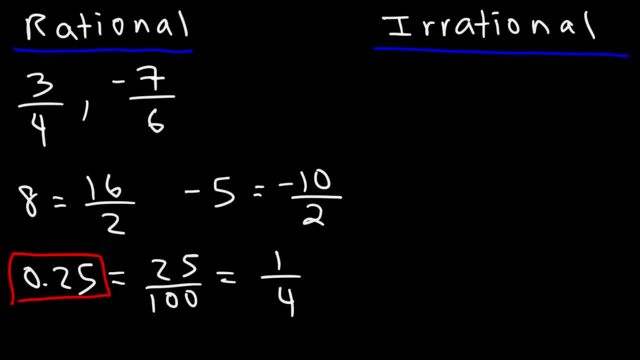 So if you have a decimal number that is finite, that comes to an end, like 0.25, that's a rational number. Another example: 0.25 is 0.15.. This you can write that as 15 divided by 100.. 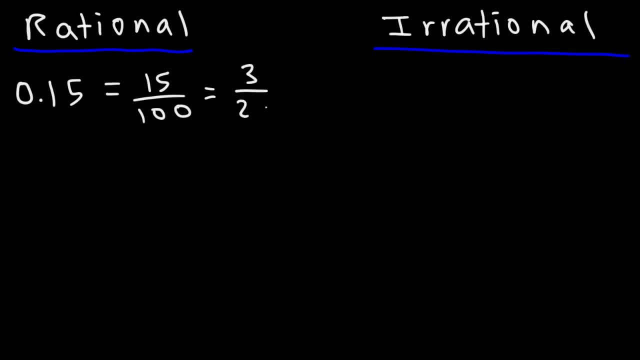 And if you divide the top and the bottom numbers by 5, you can reduce that to 3 over 20.. Now, what about repeating decimals, For instance? let's say if we have 0.6666 repeating Which we can write as 0.6666.. 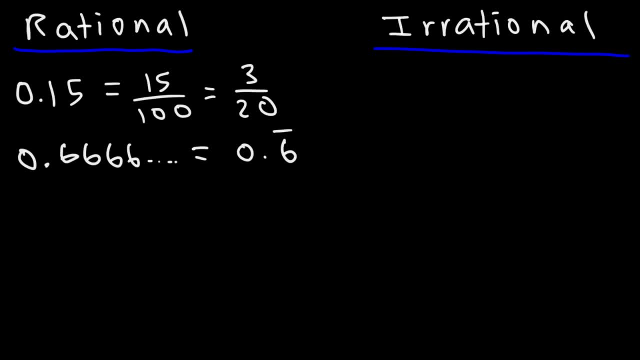 0.6 with a line on top. Is that rational or irrational? 0.6 repeating is 6 over 9, which you can reduce that to 2 over 3, if you divide by 3. So repeating decimals are irrational numbers. 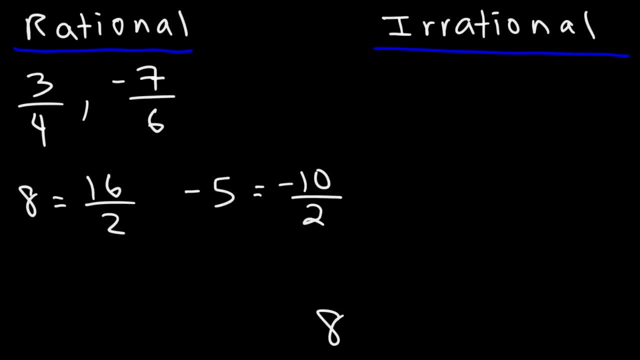 integers, then you can write it as negative ten divided by two, So negative five is a rational number. In fact, all integers are rational numbers. Now what about let's say, decimal numbers, For instance 0.25.. Is that rational or irrational? Can we write this? 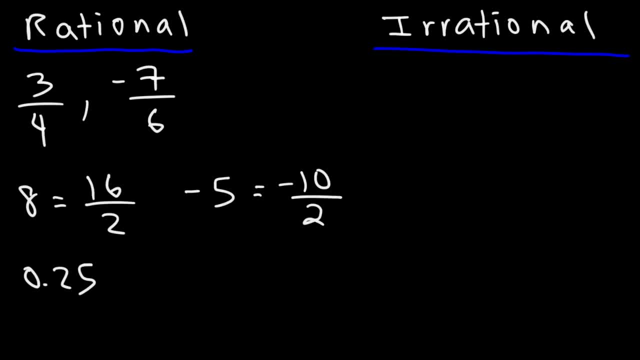 as a fraction using two integers. point 25 is the same as 25 divided by 100, and if you divide the top and the bottom number by 25, this is the same as 1 over 4. so if you have a decimal number that is finite, that comes to an end like point 2, 5, that's a. 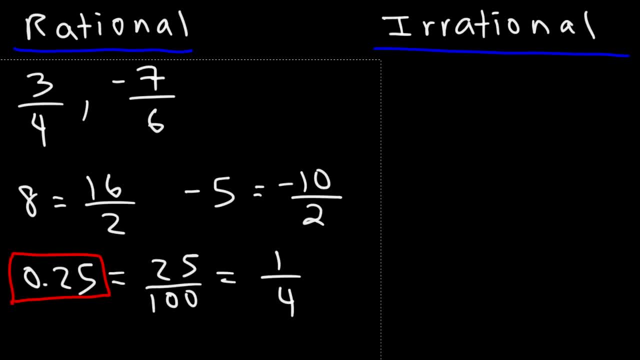 rational number. another example is point 15. this you can write that as 15 divided by 100, and if you divide the top and the bottom numbers by 5, you can reduce that to 3 over 20. now, what about repeating decimals, for instance? let's: 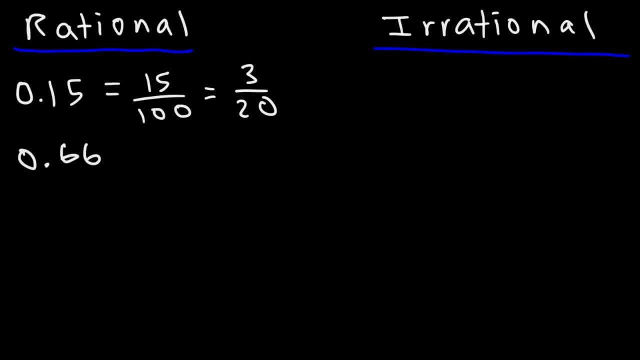 say, if we have point six, six, six, six, repeating, which we can write as point six with a line on top, is that rational or irrational? point six repeating is six over nine, which you could reduce that to two over three if you divide by three. so repeating decimals are irrational. 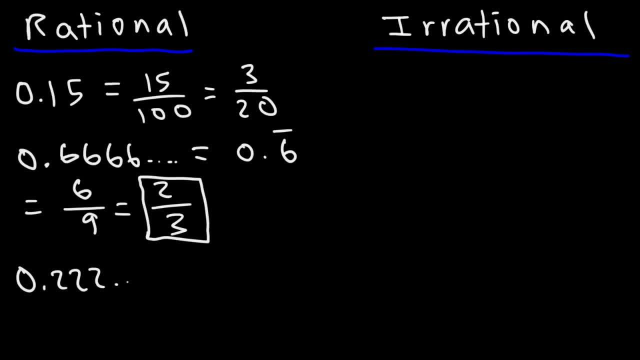 numbers. another example is point two: repeating this is two over nine. now what about let's say point 17 repeating? is that a rational number? in this case, we can write it as a ratio of two integers. point 17 repeating is 17 over 99. so whether you have a finite, 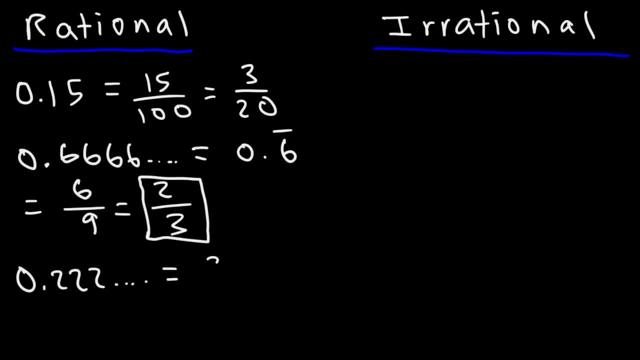 Another example is 0.2 repeating. This is 2 over 9.. Now what about, let's say, 0.17 repeating? Is that a rational number? In this case, we can write it as a ratio of two integers. 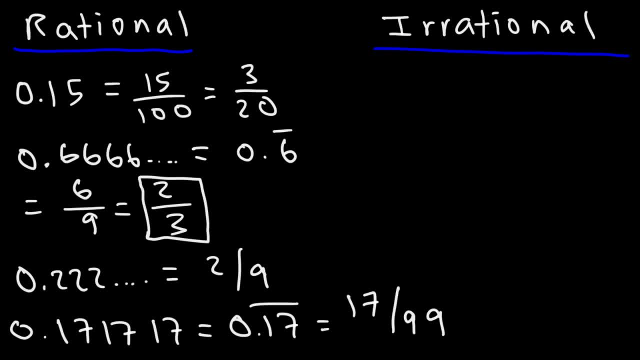 0.17. repeating is 17 over 99.. So, whether you have a finite decimal number or one that goes on forever but repeats, they're all rational numbers. Now, what about square roots, For instance the square root of 9, would you say it's rational or irrational? 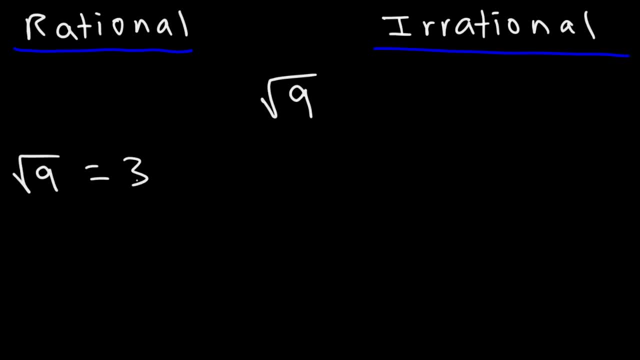 The square root of 9 is 3, and 3 is an integer, and all integers are rational numbers. But now what about the square root of 7? Is it rational or irrational? We can't simplify the square root of 7 to a whole number. 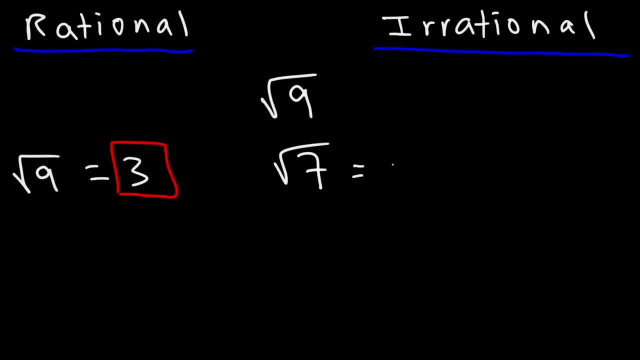 So if you use a calculator, you'll find that the square root of 7 is 2.64575131, and this can go on for a long time. So whenever you see a decimal number that is non-repeating and that goes on forever. 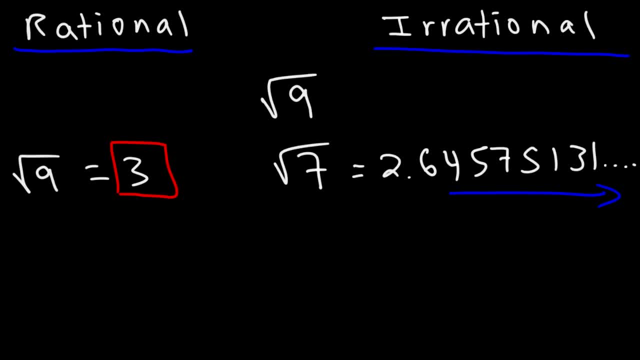 and if you can't write it as a fraction of two integers, that's when you have an irrational number. So one way to identify them is if you have a square root that can't be simplified to an integer. Typically that's an irrational number. 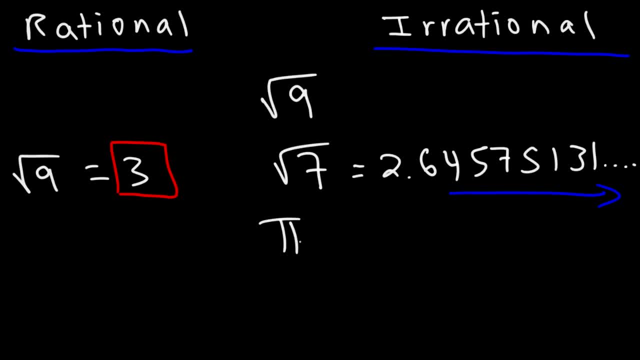 Now what about pi? Is pi rational or irrational? So if you type pi into your calculator, you're going to get a decimal number that looks like this: 3.14159265, and this also goes on. So pi is an irrational number. 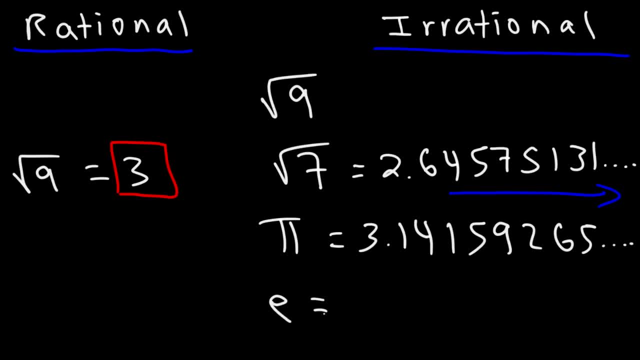 Another example is the number e. If you get the decimal value for that, it's 2.71828182, and so forth. So that's how you can identify irrational numbers. It's basically numbers with an infinite number of decimal places. 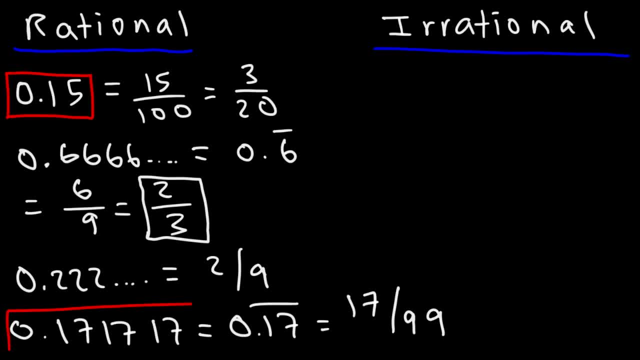 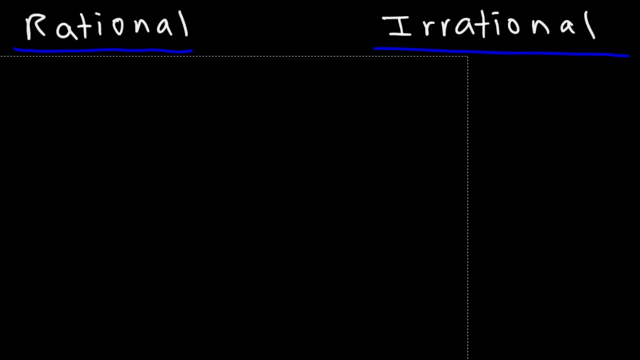 decimal number, or one that goes on forever but repeats. they're all rational numbers. now what about square roots, for instance the square root of nine, would you say. it's a rational or irrational. the square root of nine is three, and three is an integer, and all integers are rational numbers. but now what about the square? 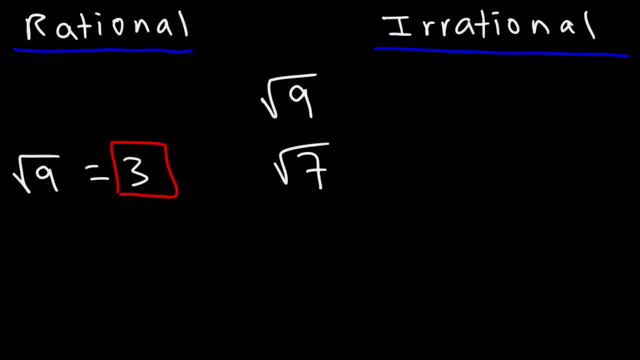 root of seven. is it rational or irrational? we can't simplify the square root of seven to a whole number. so if you use a calculator, you'll find that the square root of seven is two point, six, four, five, seven, five one, three, one, and this can go on for a long time. 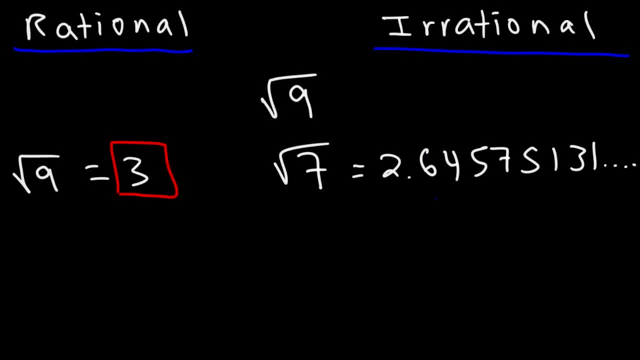 so whenever you see a decimal number that is non-repeating and that goes on forever, and if you can't write it as a fraction of two integers, that's when you have an irrational number. so one way to identify them is if you have a square root. that 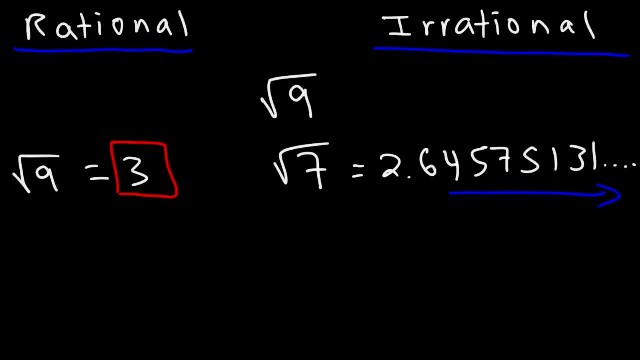 can't be simplified to an integer. typically that's an irrational number. now what about pi? is pi rational or irrational? so if you type pi into your calculator, you're going to get a decimal number that looks like this: three point one, four, one, five, nine, two, six, five, and this also goes on. so pi is an irrational. 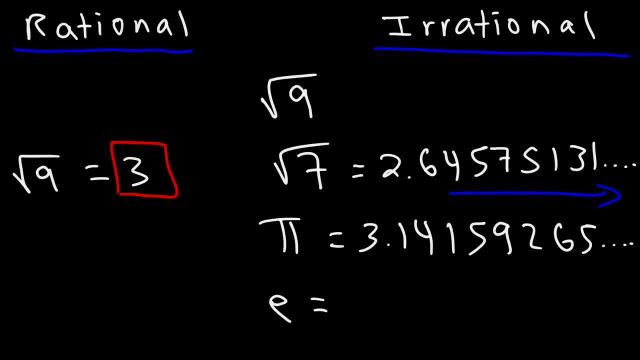 number. another example is the number e. if you get the decimal value for that, it's 2.71828182 and so forth. so that's how you can identify irrational numbers. it's basically numbers with an infinite number of decimal places. it goes on forever and you can't write it as a 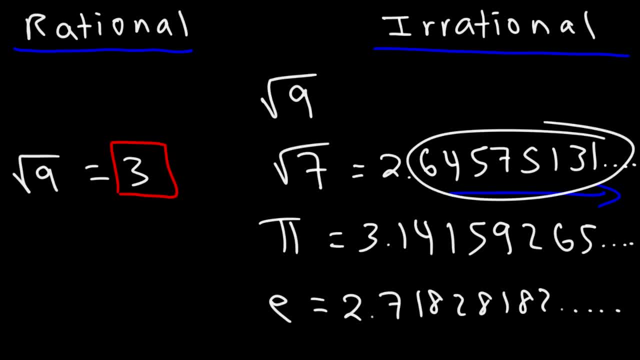 ratio of two integers. and so that's basically it for this video. now you know how to identify a rational number number and an irrational number. thanks again for watching and don't forget to subscribe to this channel.